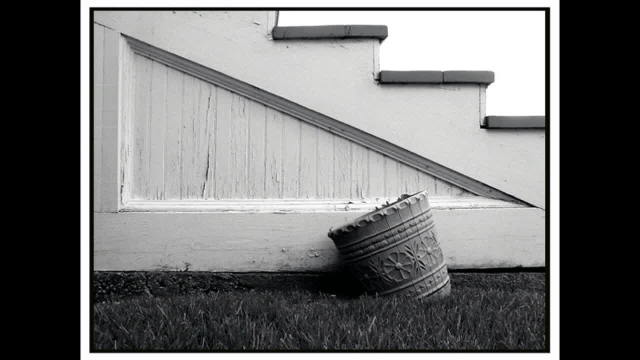 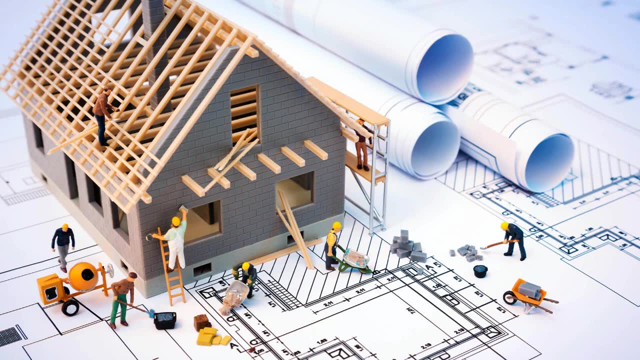 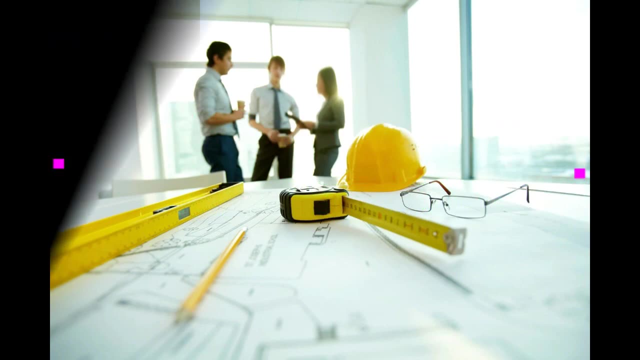 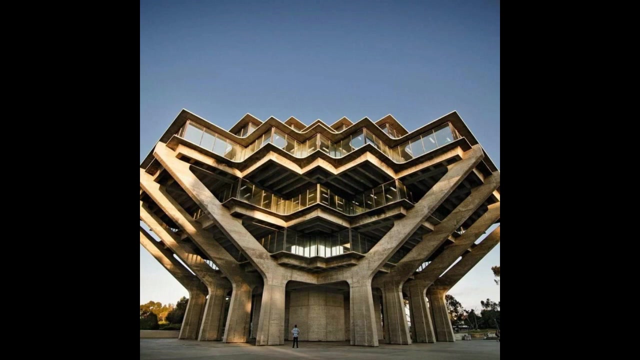 Being able to find the length of a side, given the lengths of the two other sides, makes the Pythagorean Theorem a useful technique for construction and navigation. Architecture and Construction: The Pythagorean Theorem allows you to calculate the length of the diagonal connecting the two parallel lines. This application is frequently used in architecture. 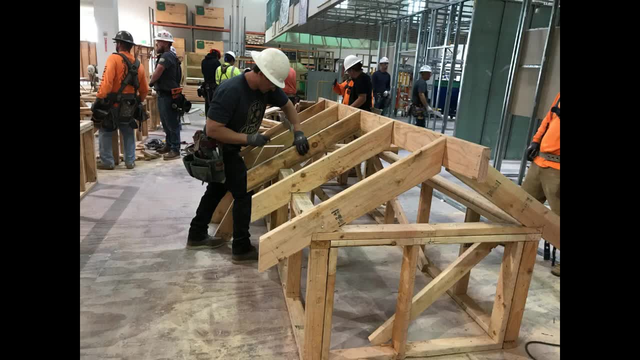 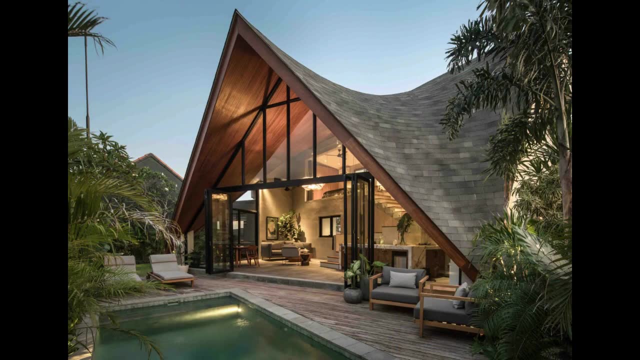 woodworking or other physical construction projects. For instance, say you are building a slope roof. If you know the height of the roof and the length for it to cover, you can use the Pythagorean Theorem to find the diagonal length of the roof slope. 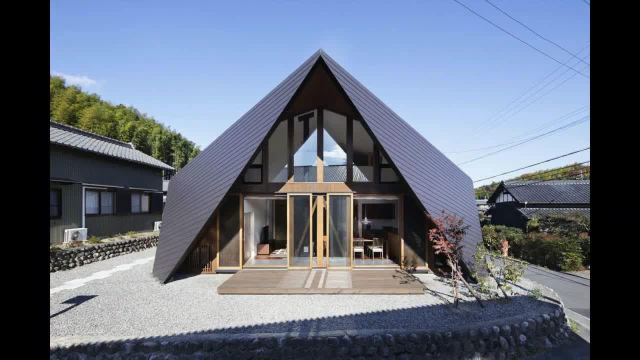 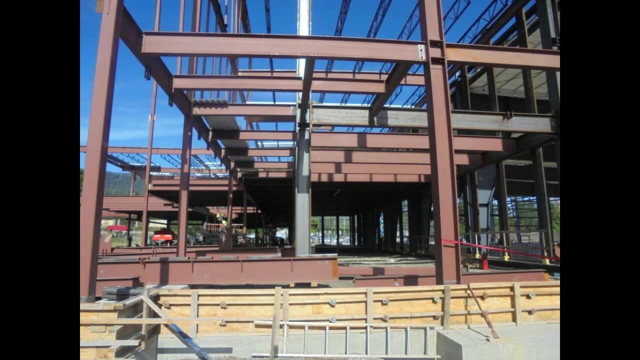 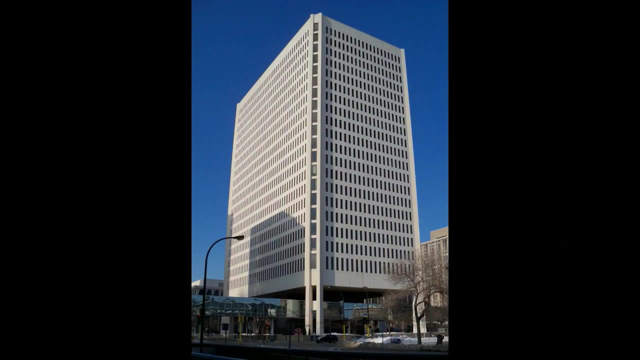 You can use this information to cut properly sized beams to support the roof or calculate the area of the roof that you would need to shingle Laying out Square Angles. The Pythagorean Theorem is also used in construction. The Pythagorean Theorem is used in construction to make sure buildings are square. 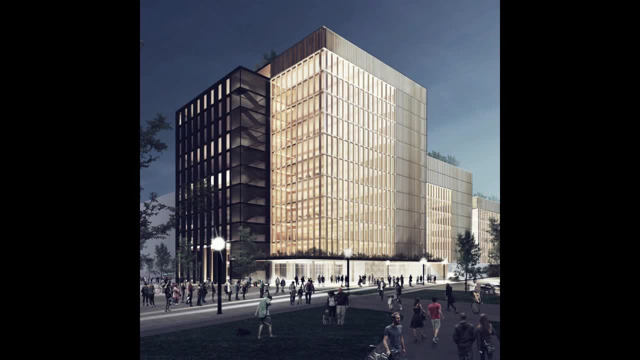 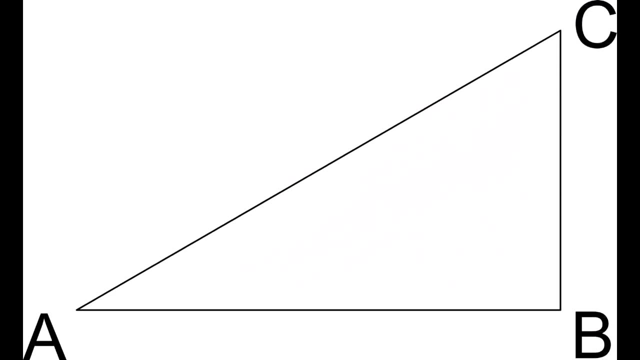 The Pythagorean Theorem is used in construction to make sure buildings are square. A triangle whose side lengths correspond with the Pythagorean Theorem, such as a 3' x 4' x 5' triangle, will always be a right triangle. 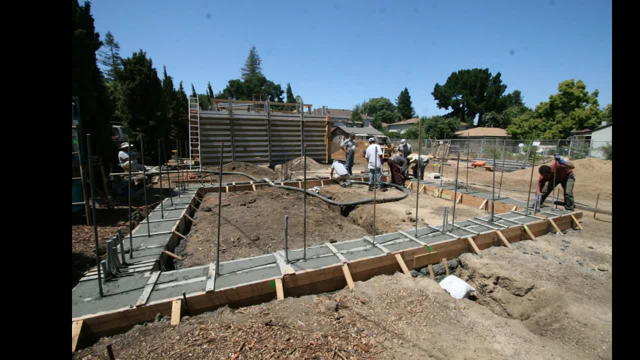 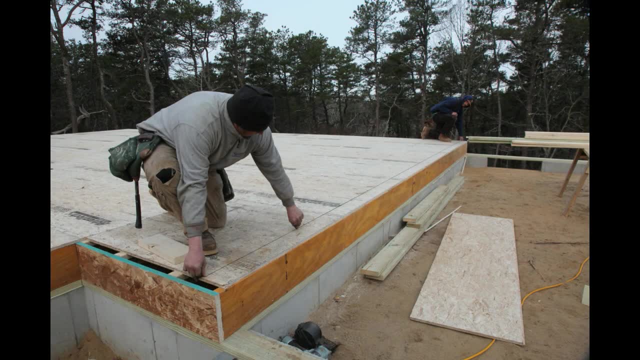 When laying out a foundation or constructing a square corner between two walls, construction workers will set out a triangle from three strings that correspond with these lengths. If the string lengths were measured correctly, the corner opposite the triangle will be the right triangle. If the string lengths were measured correctly, the corner opposite the triangle will be the right triangle. 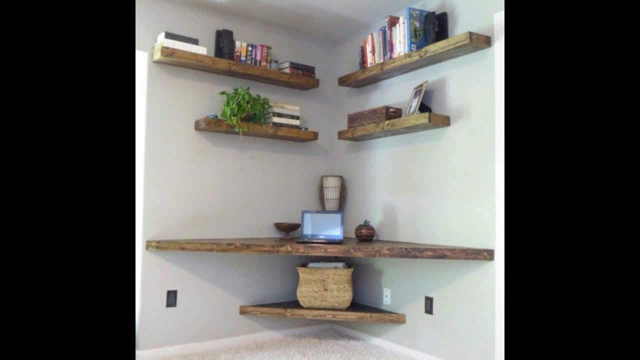 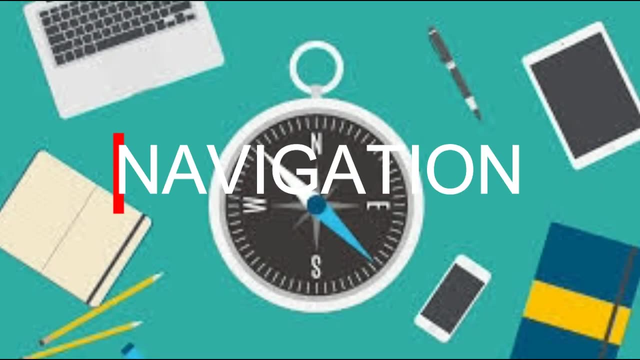 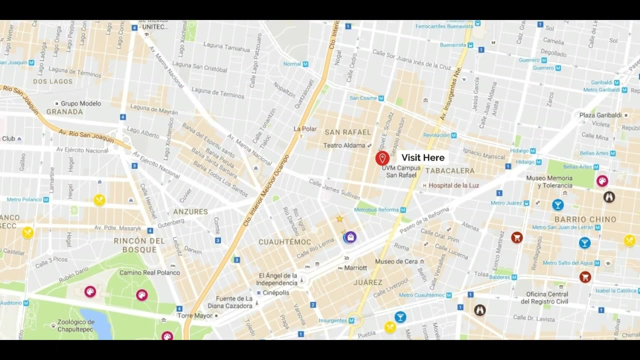 If the string lengths were measured correctly, the corner opposite the triangle will be the right triangle, So the builders will know they are constructing their walls or foundations on the right lines Navigation. The Pythagorean Theorem is useful for two-dimensional navigation. You can use it with two lengths to find the shortest distance. 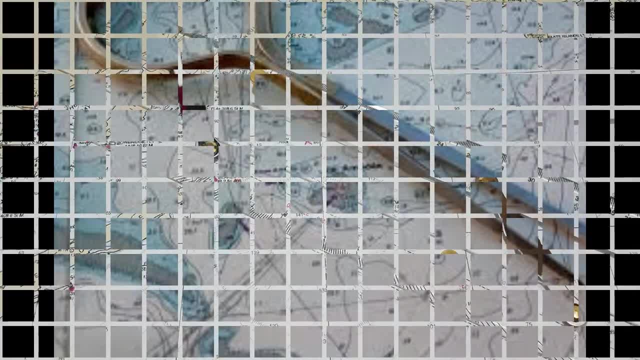 For instance, if you are at sea and navigating to a point that is 300 miles north and 400 miles west, you can use it with two lengths to find the shortest distance. For instance, if you are at sea and navigating to a point that is 300 miles north and 400 miles west. you can use it with two lengths to find the shortest distance. For instance, if you are at sea and navigating to a point that is 300 miles north and 400 miles west, you can use it with two lengths to find the shortest distance. 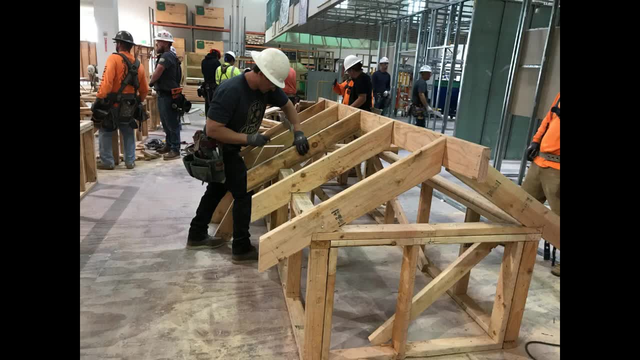 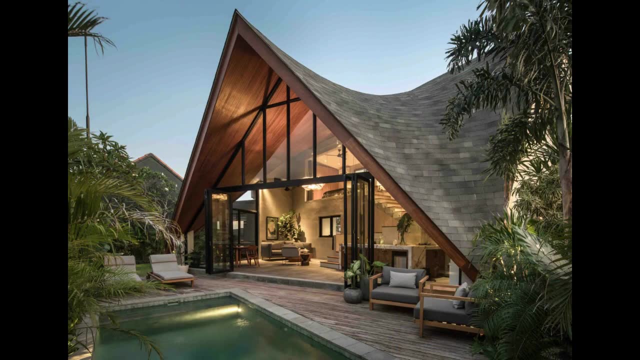 woodworking or other physical construction projects. For instance, say you are building a slope roof. If you know the height of the roof and the length for it to cover, you can use the Pythagorean Theorem to find the diagonal length of the roof slope. 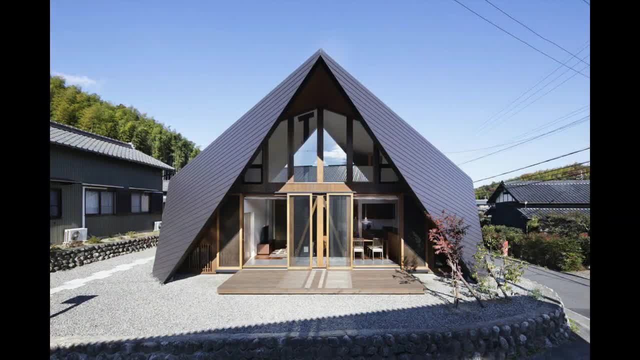 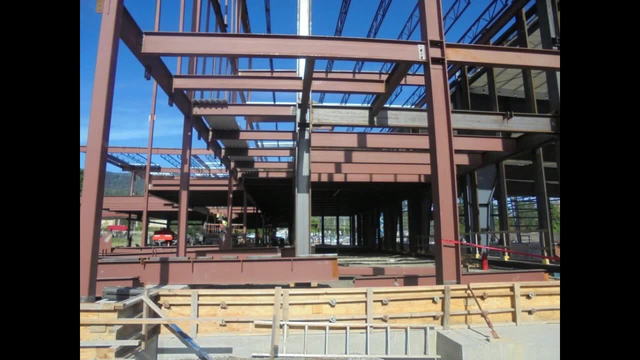 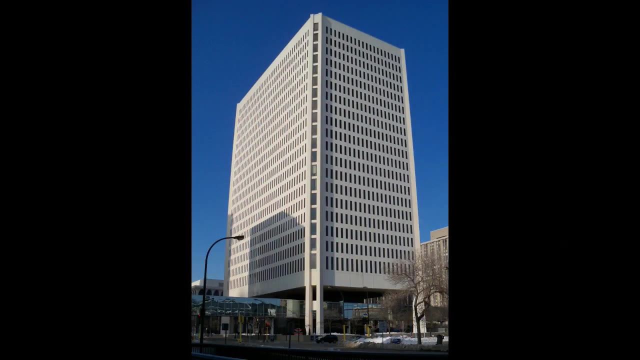 You can use this information to cut properly sized beams to support the roof or calculate the area of the roof that you would need to shingle Laying out Square Angles. The Pythagorean Theorem is also used in construction. The Pythagorean Theorem is used in construction to make sure buildings are square. 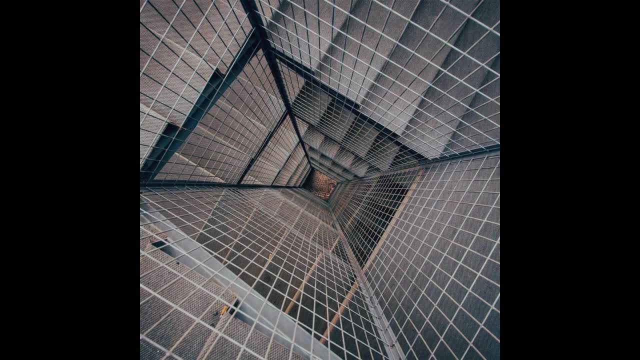 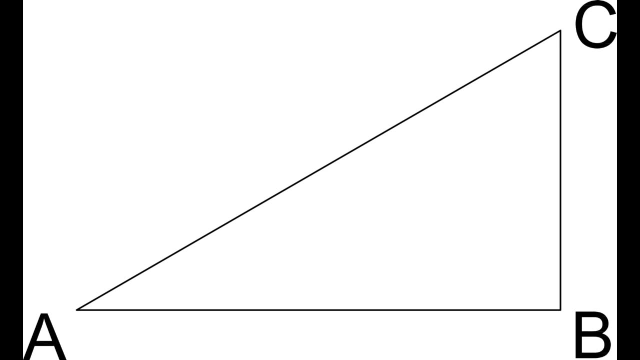 A triangle whose side lengths correspond with the Pythagorean Theorem, such as a 3' x 4' x 5' triangle, will always be a right triangle When laying out a foundation or constructing a square corner between two walls. 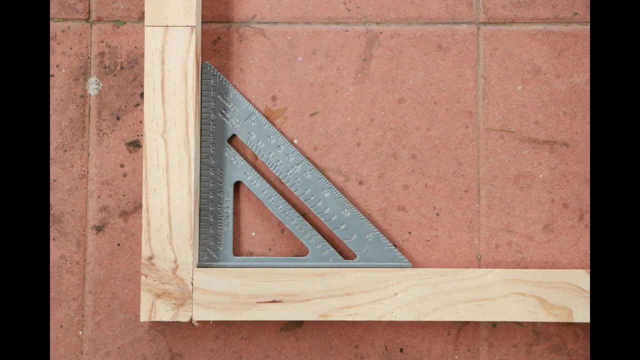 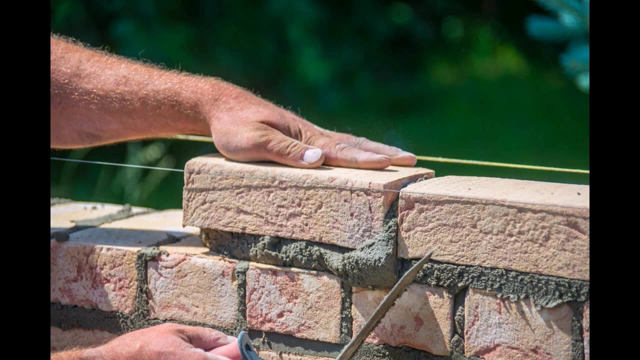 construction workers will set out a triangle from three strings that correspond with these lengths. If the string lengths were measured correctly, the corner opposite the triangle will be a square. If the string lengths were measured correctly, then the corner opposite the triangle will be a right angle. 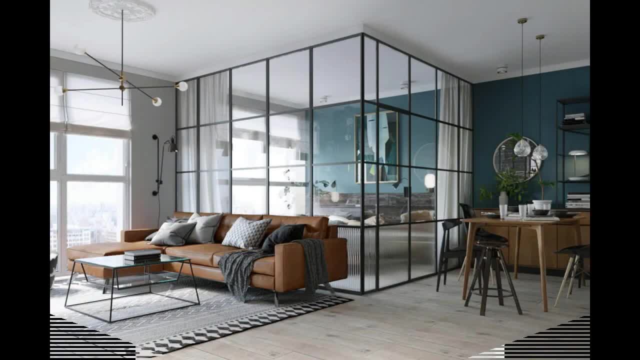 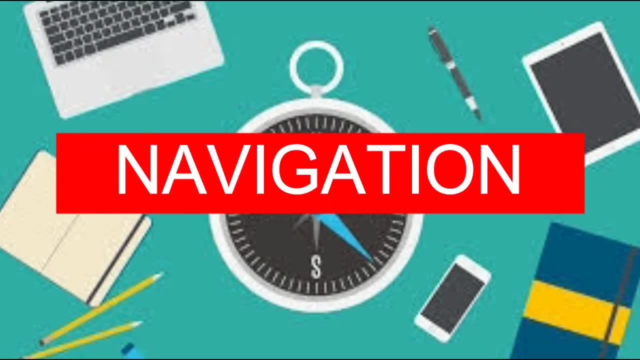 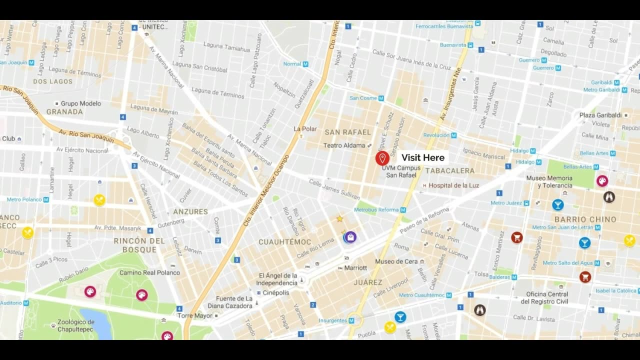 So the builders will know they are constructing their walls or foundations on the right lines. Navigation: The Pythagorean Theorem is useful for 2-dimensional navigation. You can use it with two lengths to find the shortest distance, For instance, if you are at sea and navigating to a point that is 300 miles north and 400 miles south. 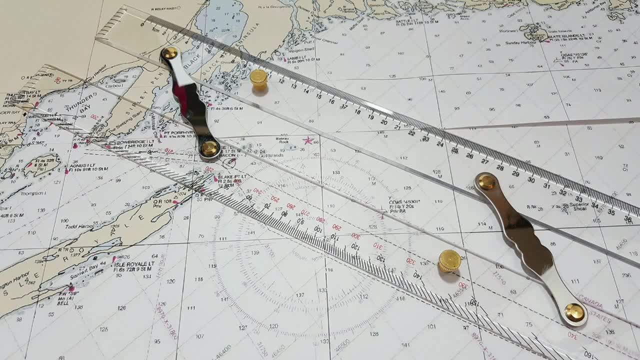 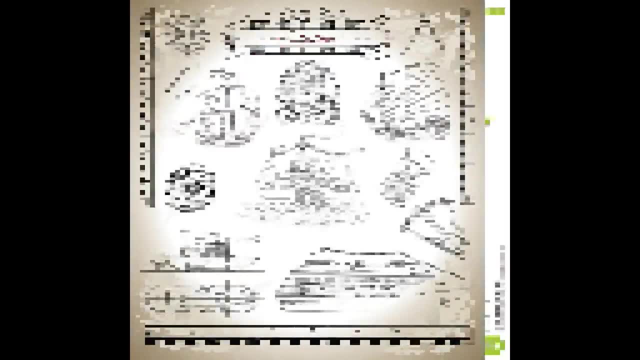 you can use this information to determine the longest distance to the table west. You can use the theorem to find the distance from your ship to that point and calculate how many degrees to the west of north you would need to follow to reach that point. The distances north. 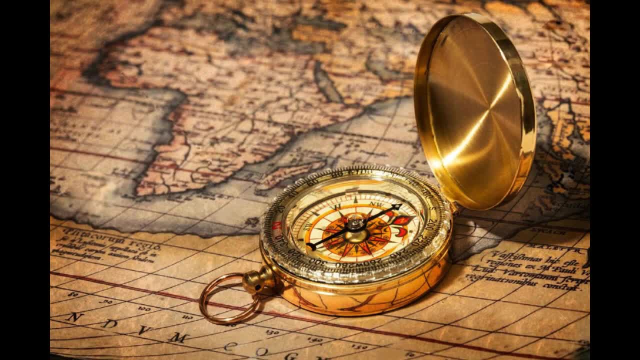 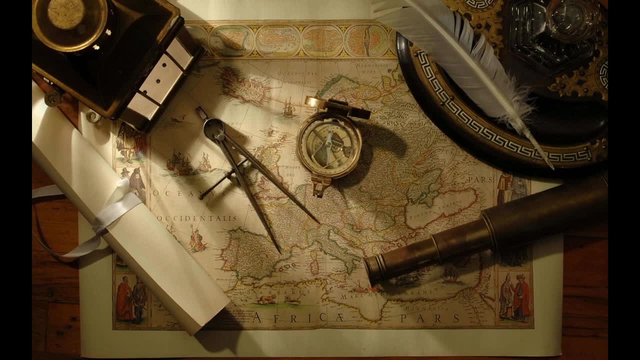 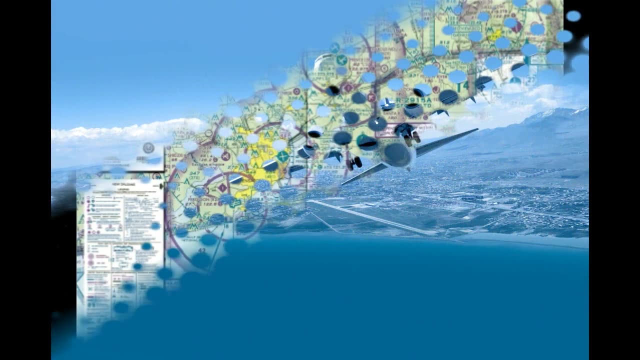 and west will be the two legs of the triangle, and the shortest line connecting them will be the diagonal. The same principles can be used for air navigation. For instance, a plane can use its height above the ground and its distance from the destination airport to find the correct place to